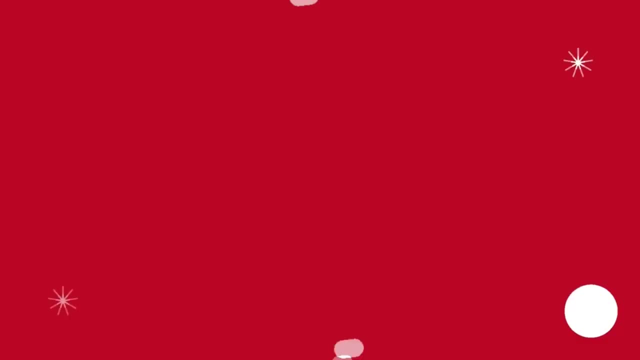 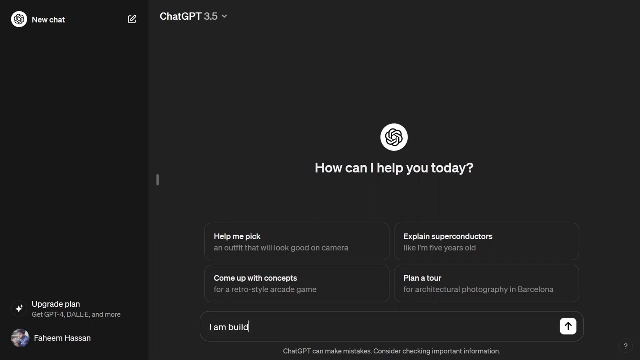 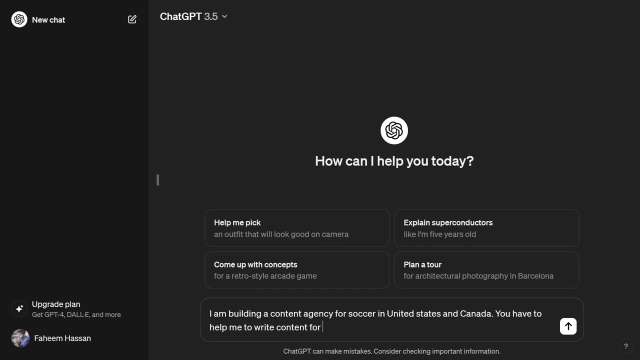 contact form. So, without any delay, let's start. Okay, first of all, I will provide a context again. like I'm building a content agency for soccer in United States and Canada, You have to help me to write content for the whole page of my website that I want to develop. So, first of all, provide me content of the whole page. 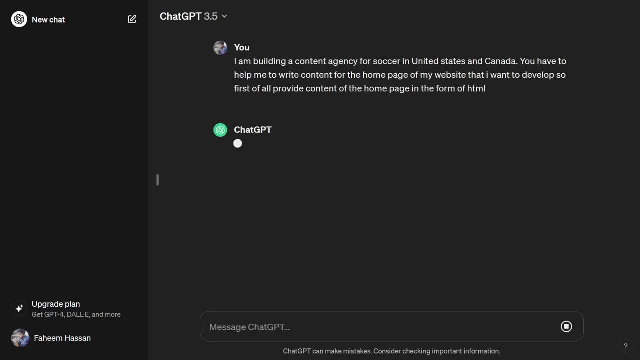 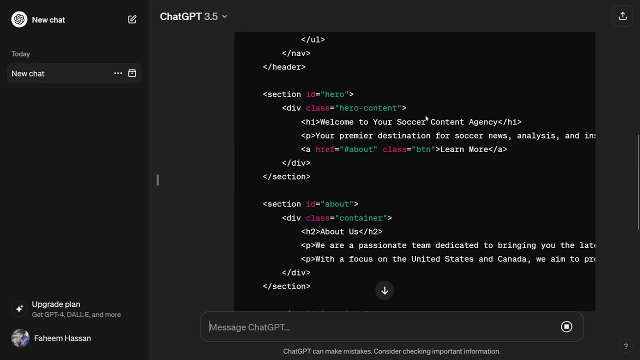 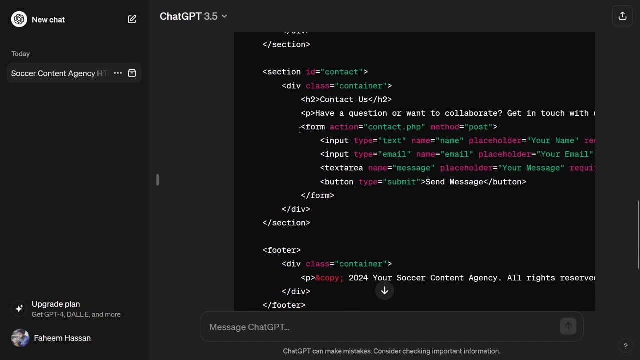 in the form of html. Let me press enter. So here was my prompt and you can see that it is providing me the content of my home page about page, our services and contact us. You can see that it is also provide me a contact form here and in the last it have. 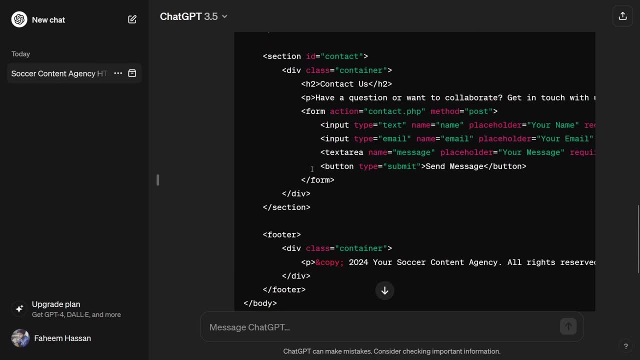 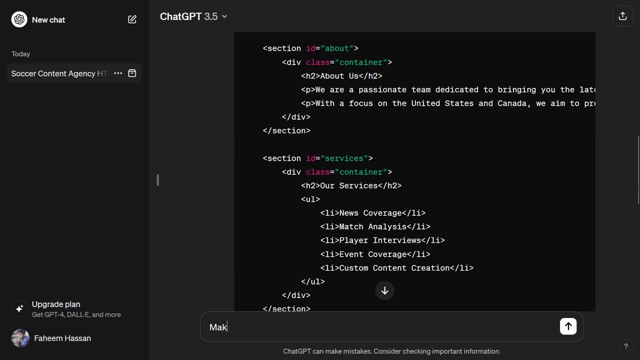 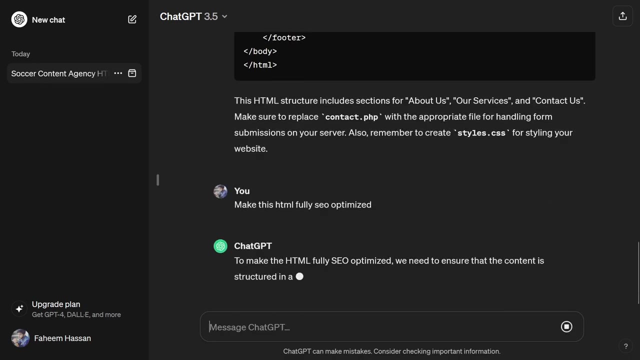 provided me this html, So you can see that we can get html for our website. Okay, now let me type another thing. for example, make this html fully SEO optimized. Let me press enter again and friends, now you can see that before this chat: gpt, do not. 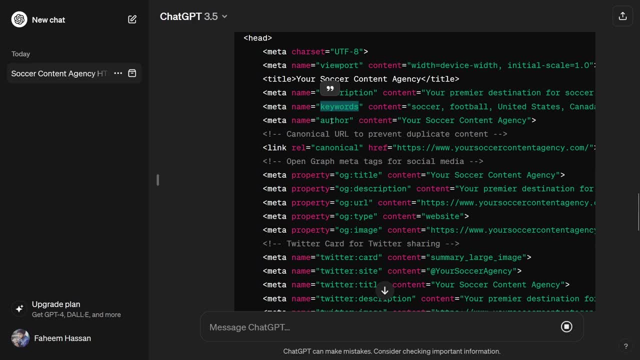 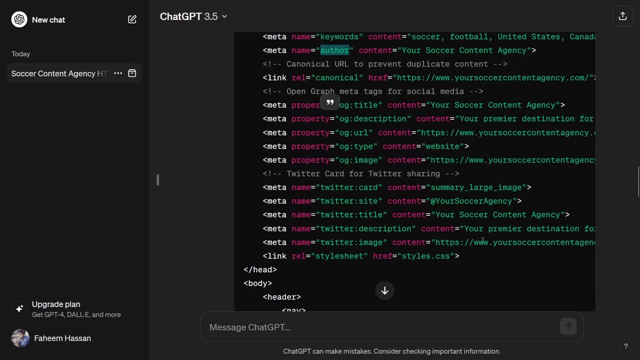 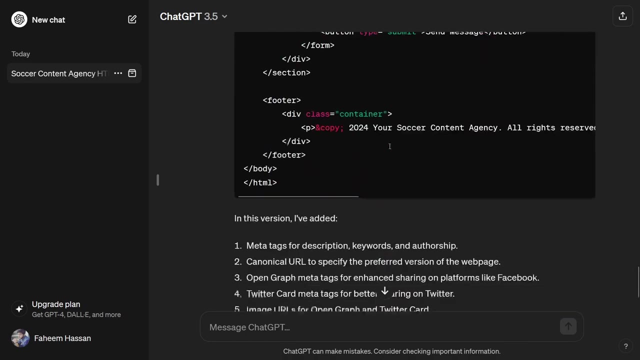 add this type of stuff like description, keywords, author, and. but now you can see that because I have asked chat gpt to write SEO friendly page for me, So it is also providing me SEO friendly page here. Let me scroll down and this is the content of our html. Obviously, the people's who now SEO content of our html. So I will be adding SEO page as my facebook page, and the people's who now SEO placed my content as SCO friendly page, So it is also providing me SEO friendly page here. Let me scroll down and this is the content of our html. Now let me scroll down and where the person who now SEO is: 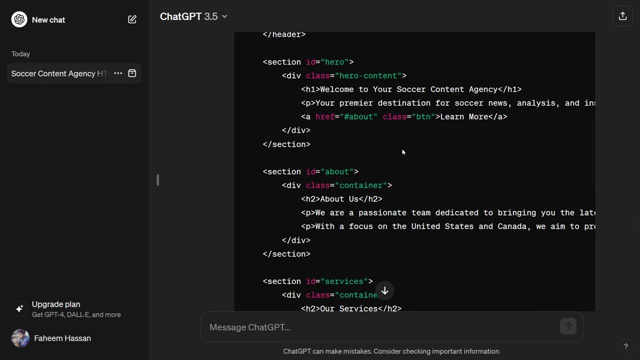 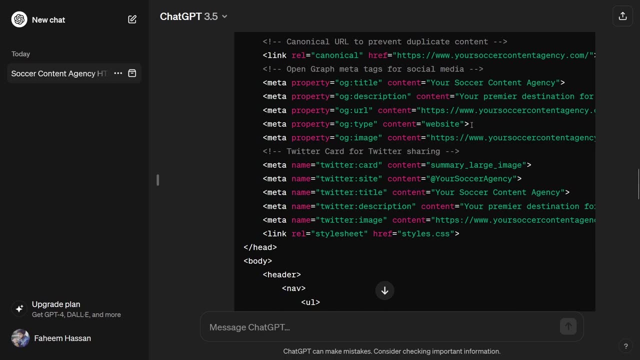 the page. I will Аmbition a page. So let me just click on here and I will try to enter a page. So for the people who now seo and who are also watching this video, they know that this stuff is very important from seo point of view also. you can see that it is also provides some backlinks. i know that it. 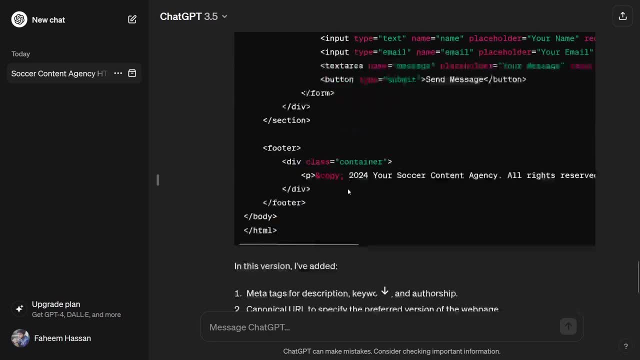 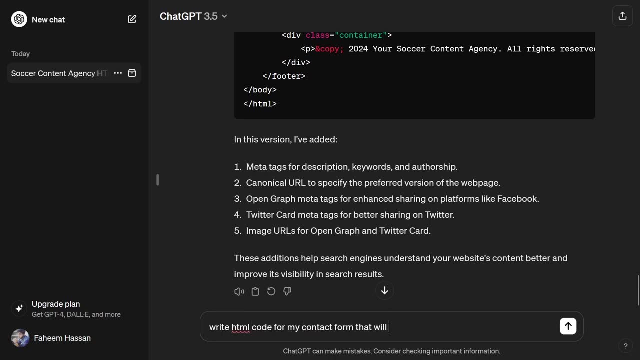 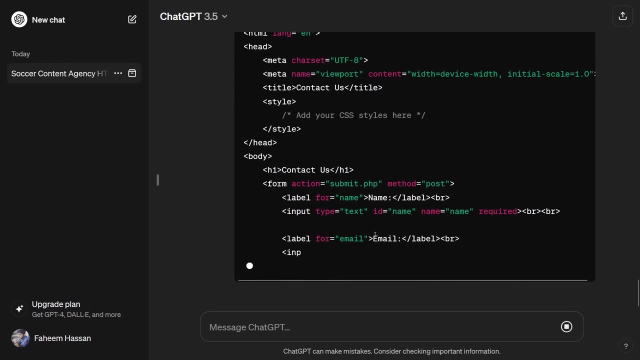 have provided us with the contact form, but let me again type here, write html code for my contact form that will get user favorite color from red, green and pink, also their name, email and their message. so provide me with the html code, so let's see what it will reply with us. so, friends, here you. 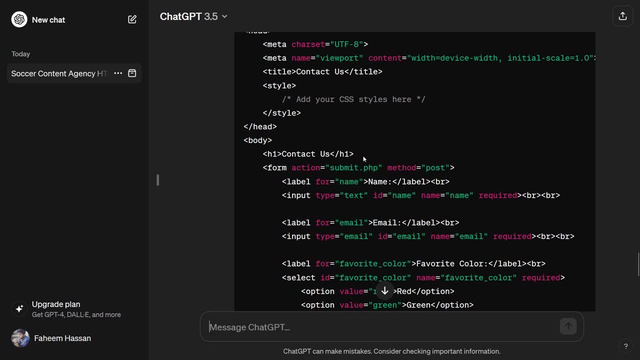 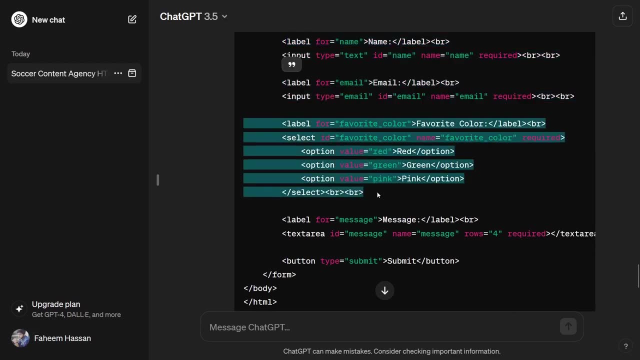 can see that. uh, now it have. create us a form for us and the and the. the first field is for name, for email, for our favorite color, a select field and another text area field to get message from the user. so all these things were mentioned in our prompt and 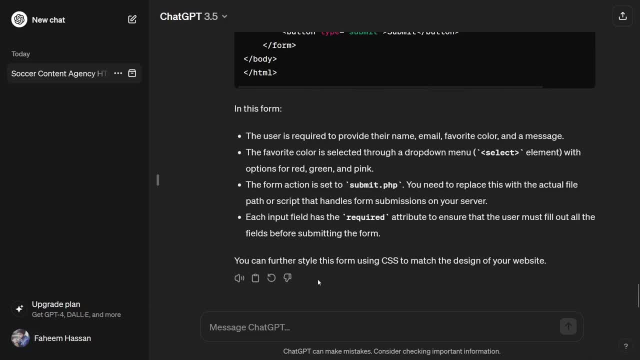 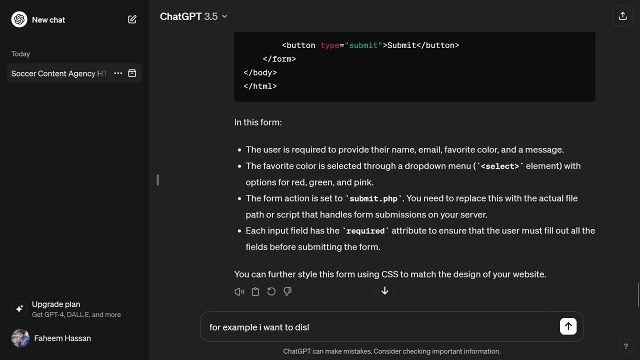 as it is chat gpt have provided us now, for example, i also want to display some content on my contact us page. okay, for example, i want to display some content on this contact us page that you have created for me. so keep in mind my niche, which is soccer, and write seo friendly. 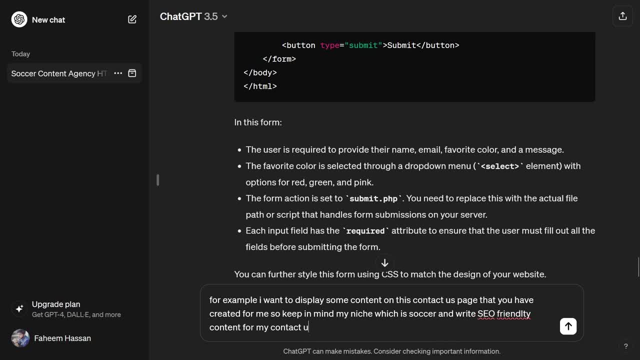 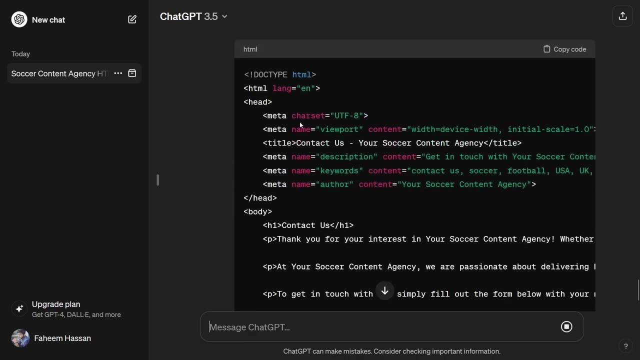 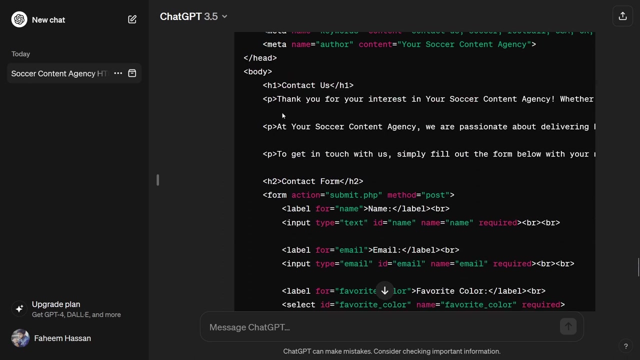 content for my contact us page. also. keep in mind that i am targeting usa and uk. for example, let me press enter and friends. now you will see that it is providing me the same page with the seo friendly content like keywords, description, author, and here you can see that. thank you for interest in soccer content agency. at your soccer content agency, we 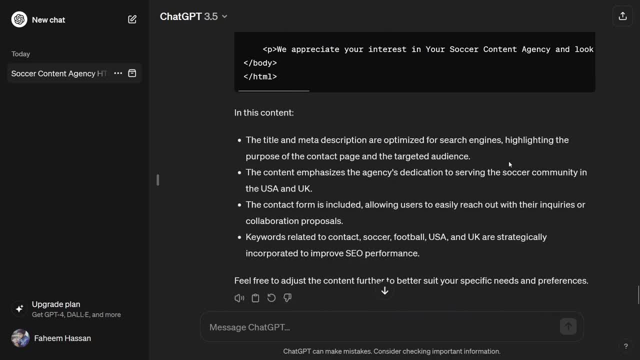 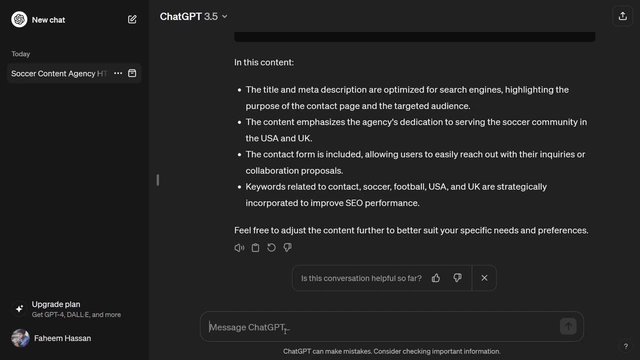 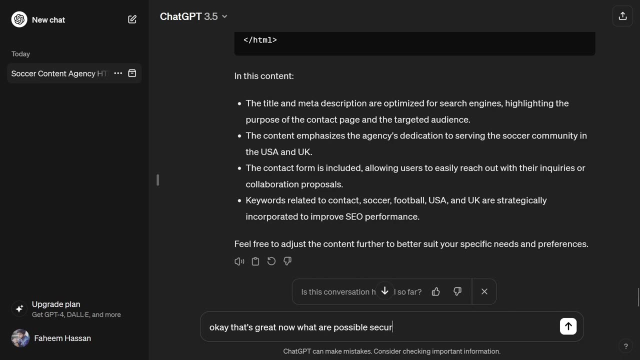 are passionate about delivering. so, hey, friends, here you can see that. and in the last, let me ask chat gpt that what are security risk in our html form? so let me type here: okay, that's great. now, what are possible security risks that html form you provided to me? can you explain that? let me press.